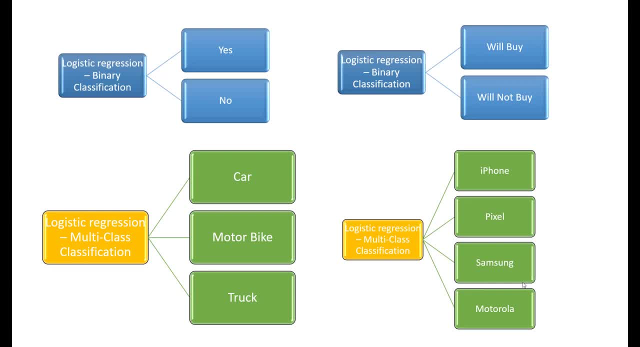 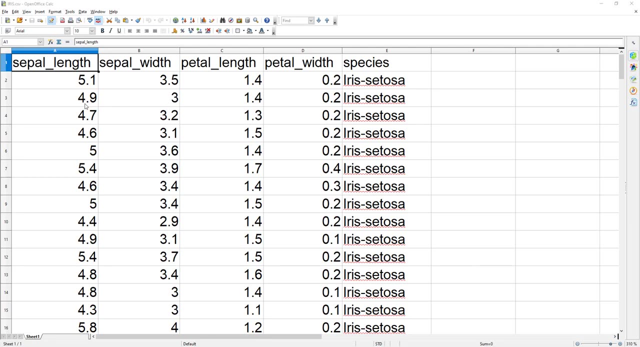 the phone is a iphone, or it is a google pixel, or it's a samsung, or it's from motorola. So these are examples of multi-class logistic regression. In this video of multi-class logistic regression, we are going to use this iris dataset. This dataset has different attributes, like sepal length. 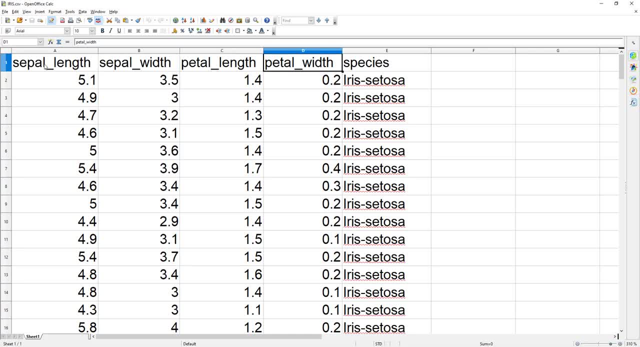 sepal width and sepal length. Petal length and petal width. Using all these attributes- these are independent variables or independent attributes. Using all these independent attributes, we are going to predict the species which is the dependent attribute, and this species has three possible values. 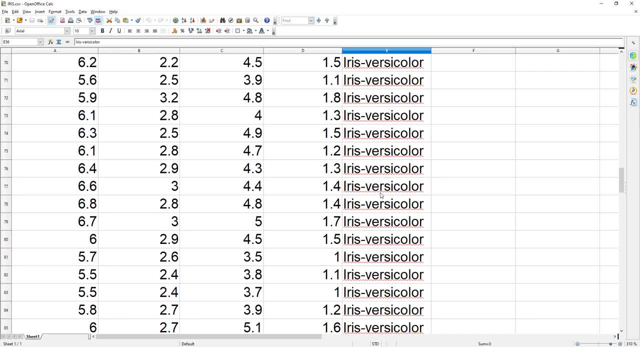 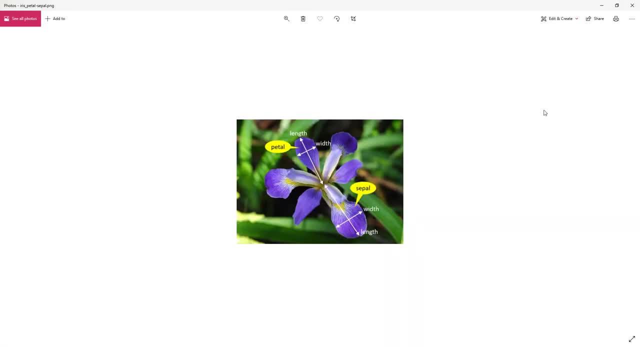 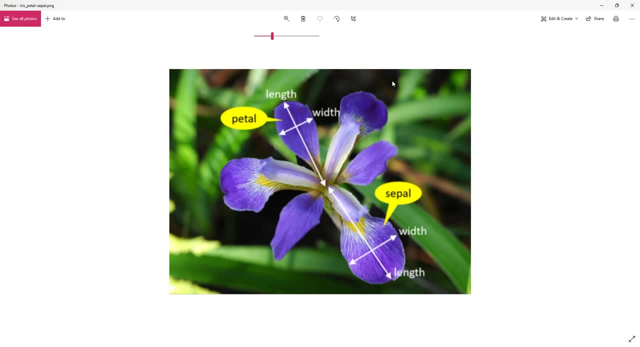 One is iris cetosa, one is iris versicolor and the next one is iris virginica. If you wanted to get a feel of what this dataset is about, iris is nothing but a flower and it has different species. This flower has different species and what we have in our dataset is the petal. So this part is the petal and we do. 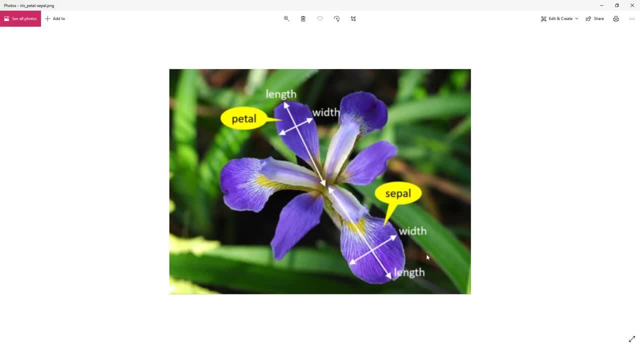 have lengths of the petal and the width of the petal and this part of the flower. it is sepal and we do have the length and width of the sepal. So, using these attributes, we are going to predict that this is a flower and that if we want to get a feel for it is that it has different species. 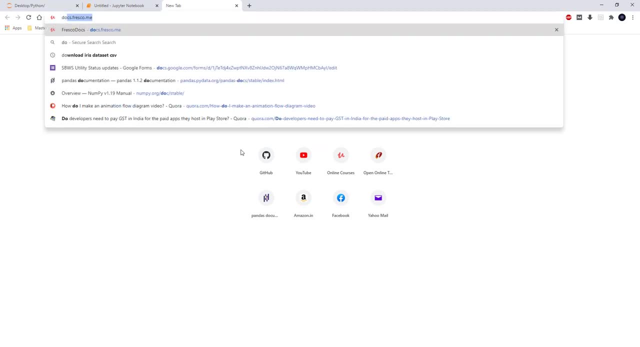 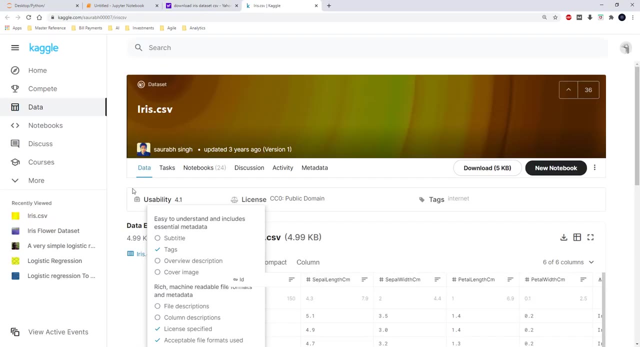 So the following is our dataset. This is how this dataset is and it has been used in our dataset. So first we are going to use a set of iris flower. The name of the flower and the type of iris is one, So we are going to use this. This is a flower with the leaves. I have downloaded this. 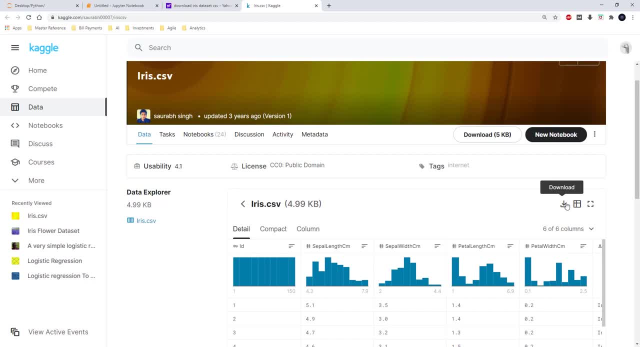 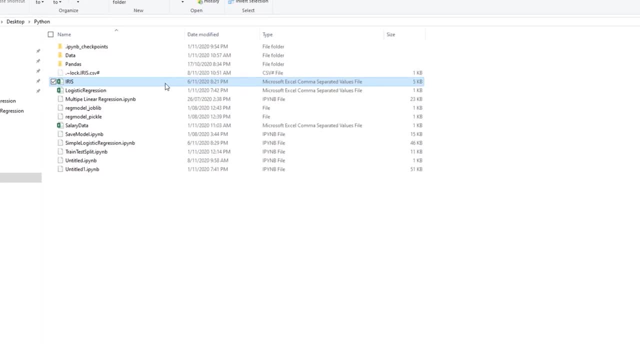 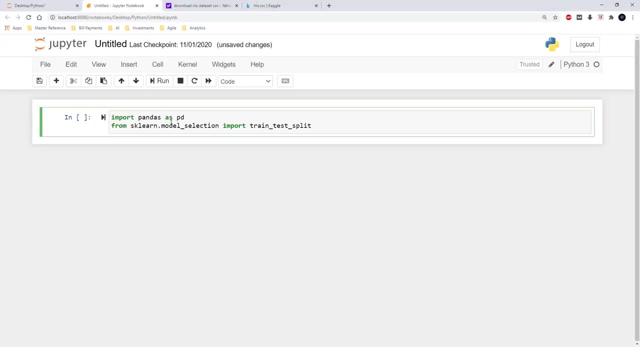 data from cagglecom use this data set, and then I just downloaded it and we are going to use it for our demo. I have downloaded this iris data set in the same location as my code and I am going to use Jupyter notebook for this demo. in the first two lines I 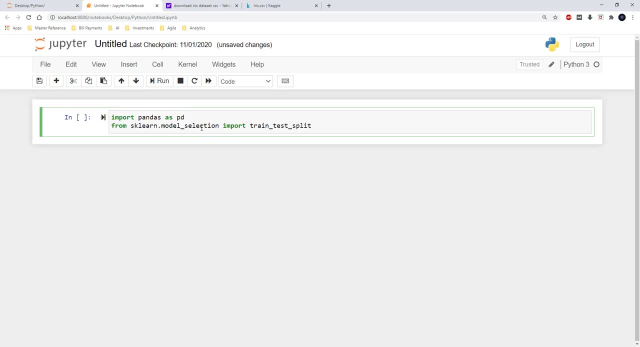 am importing pandas and from sklearn dot model selection I am importing train test split. I will run this block of code. next I am going to read the iris file that we have just downloaded and I am going to store it in a data frame by name data. once I store it, then I am going to print the data frame when I run. 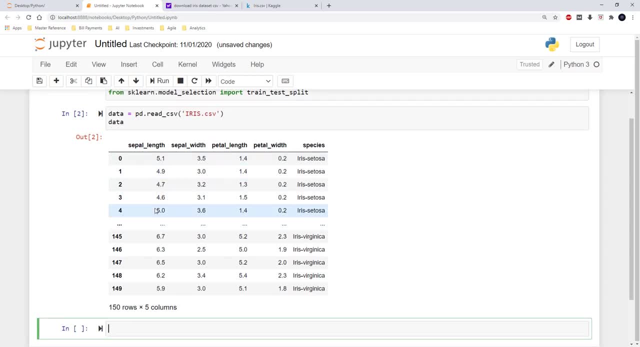 this piece of code you can see that the data is printed and here you can see that the sepal length, sepal width, petal length and petal width are displayed, and we can also see the species name displayed. so totally there are 150 rows and 5 columns. machine learning models handles only numeric data, and here we. 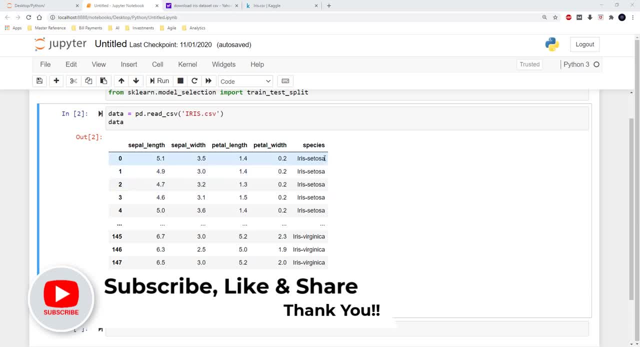 have numeric data for all the columns except for species. I wanted to change the value of each species into a number in order to do that. I just wanted to know what are all the species are available, because here in this display I am not able to see the entire value of all the species. 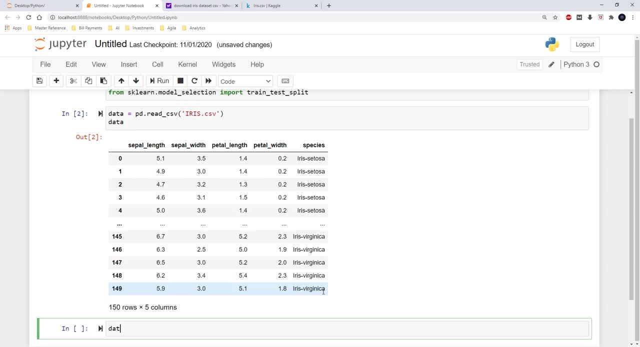 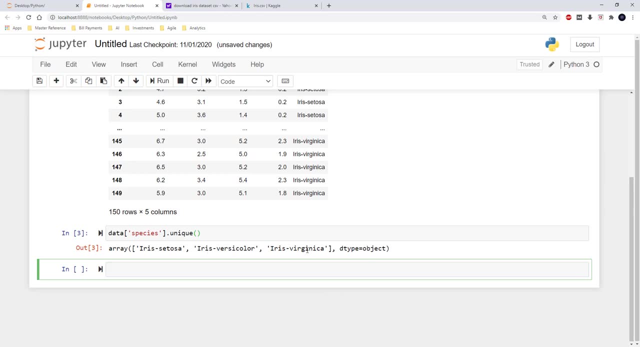 so in order to get that, I am just using data of pieces dot unique. so when I run this line, I can see that there are three unique values for species. so what I am planning to do is for iris setosa- I am going to modify this as one- and iris. 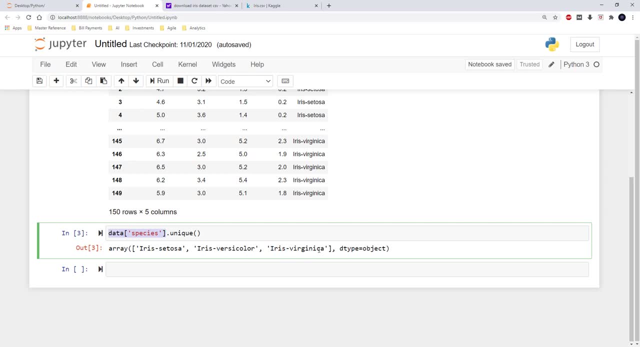 versicolor, I am going to replace it with two, and iris virginica, I am going to replace it with three. in order to do that, I am going to use replace command. so here I am going to use data species, the dot replace and within the replace I am going to give the inputs as dictionary. so in the first 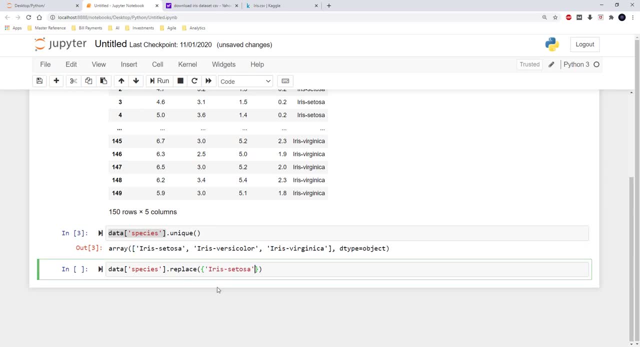 value, which is iris setosa, I am going to replace it with one, and then the second value, iris versicolor, I am going to replace it with two, and the third value, iris virginica, I am going to replace it with three. now I have done this, I am going to assign this output back. 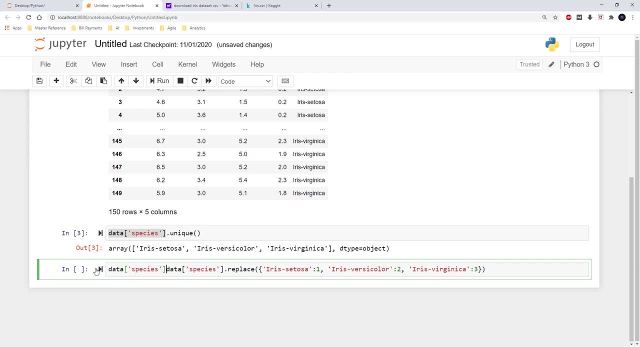 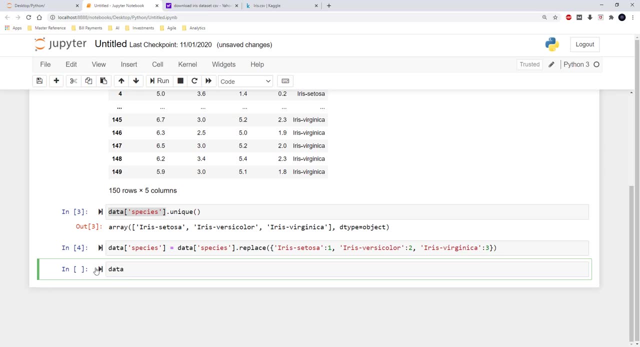 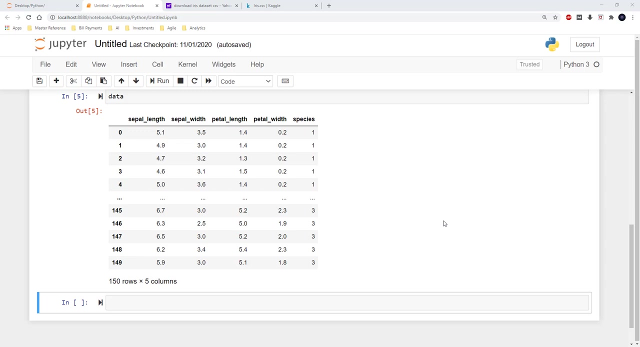 to data species, so that I can just have the change stored back. when I run this piece of code and then when I display the data again, you can see that the values from species has been replaced by one to one three. before I can create the multi-class logistic regression model, I wanted to split this data. 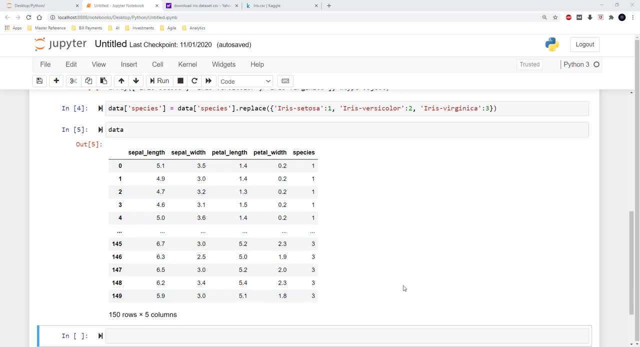 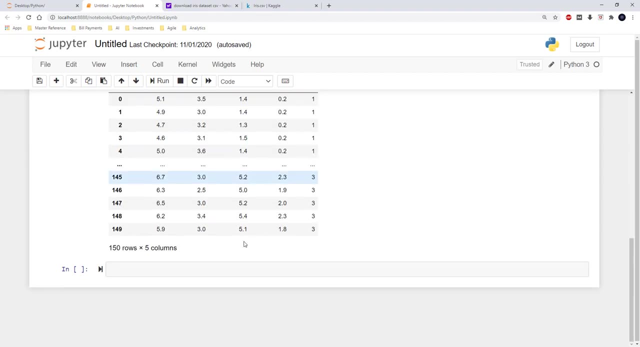 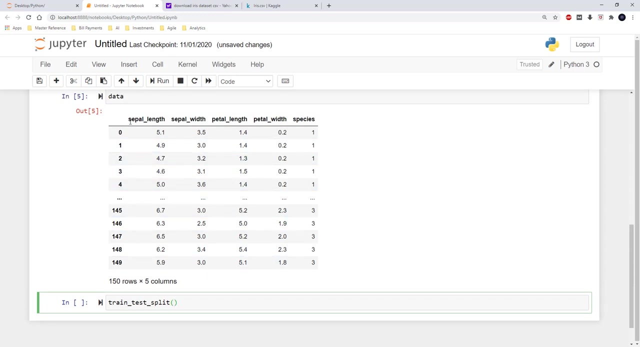 into a trading and testing data set. so in order to do that, I am going to use this train test split that we have imported earlier. so here I am using the strain test split and then I am going to just give all these independent attributes like sepal length, sepal width, petal length and petal width. 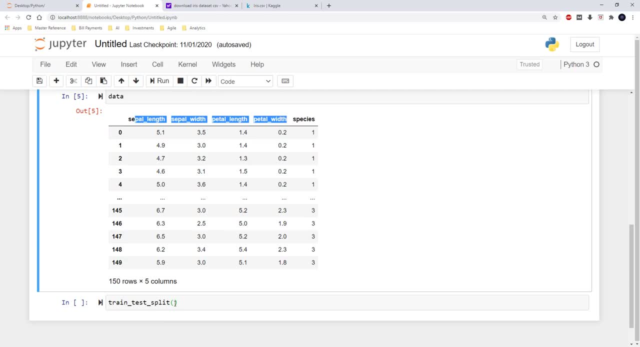 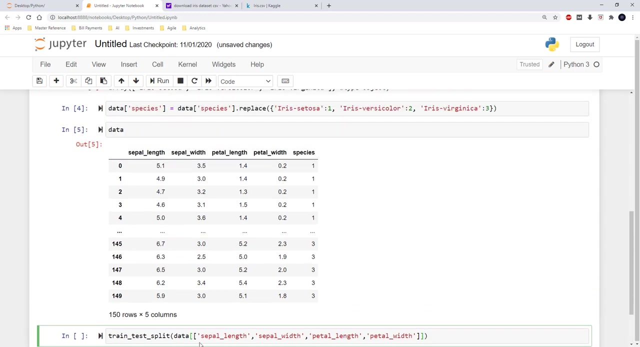 these are the independent attributes. I am going to give this as x parameter and then y parameter. I am going to give this pieces, so let me quickly do that. so in the test train split I have given the x parameter with a list of all the independent attributes, and now I am going to give 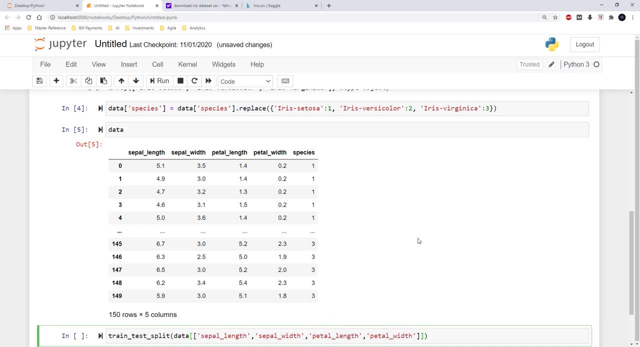 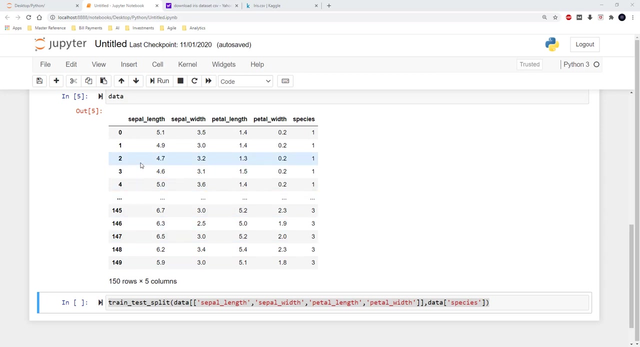 the y parameter of the test train split, which is going to be species, and this is the dependent data- has a set of independent attributes like sepal length, sepal width, petal length and petal width, and it has one dependent attribute, which is pieces. when I run this line of code for train test split: 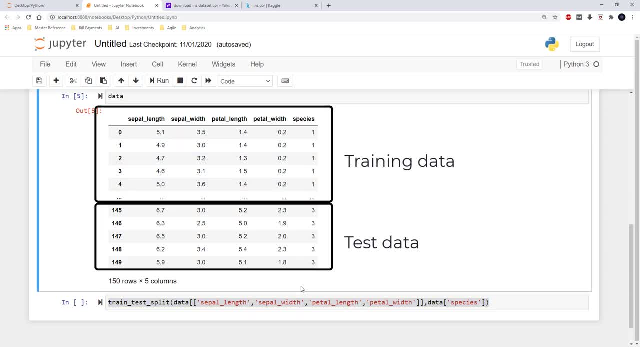 what happens is this entire data with 150 rows is split into two blocks. one block is for training and one block is for testing, and within each block there will be both independent attributes and dependent attributes. the independent attributes, we are going to name it with capital X, and the dependent attribute, we are going to name it. 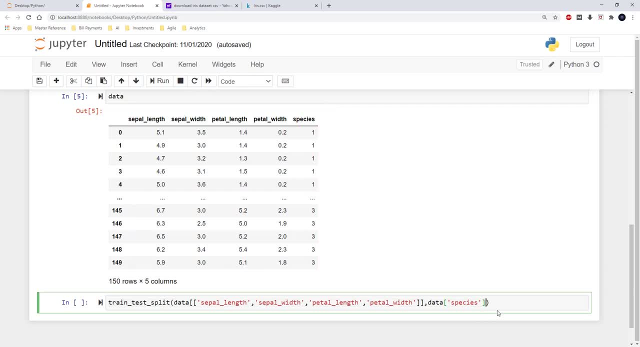 with small y and I need to specify here on how much data I need to have for testing. so I am going to specify it with test size and I am going to have twenty percent of the entire data set for testing, which means that out of 150 rows, 30 rows will go for testing and the remaining 120 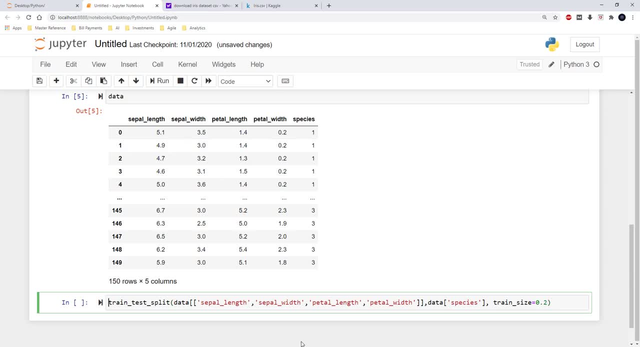 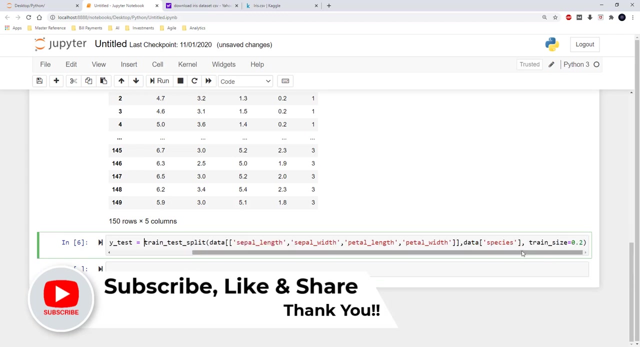 rows will be used for training and I am going to store the output of this split into x train, x test, y train and y test. so when I run this piece of code, all these variables- x train, x test, y train and y test- would have been populated. so here I have done one mistake. I wanted to specify. 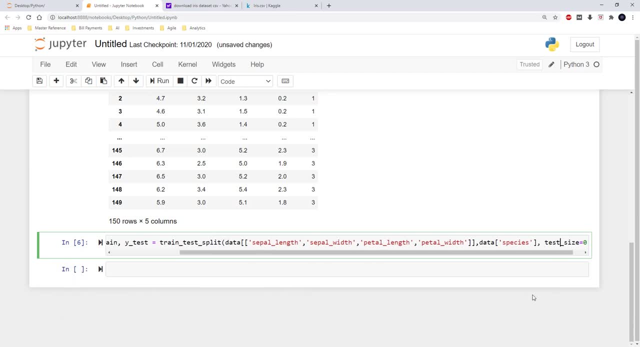 test underscore size instead of train size, because for training I will have to use 80 percent of the data and for testing I will have to use the remaining 20 percent of the data. so I will run this piece of code again for your reference, or I am going to display the training. 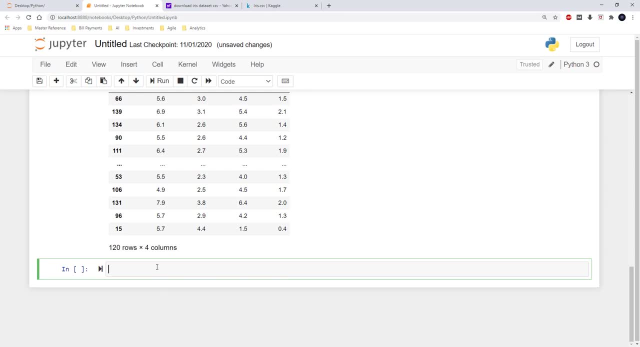 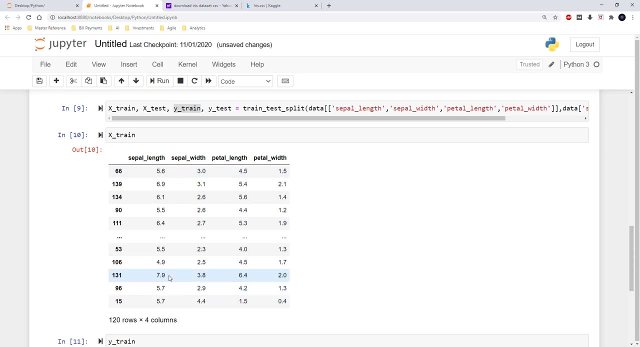 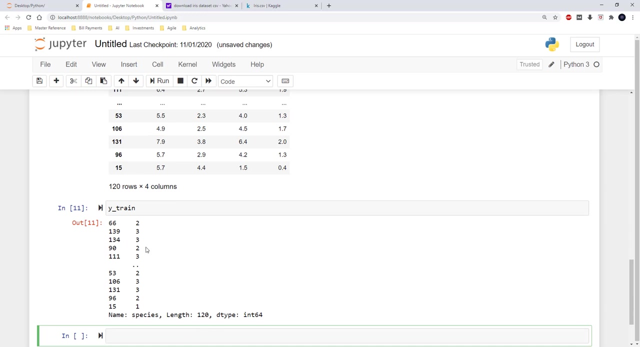 data set. so when I display the training data set, you can see that there are 120 rows and there are four columns with all the independent variables. and when I display y train, you can see that there are same 120 rows with the corresponding dependent variables for. 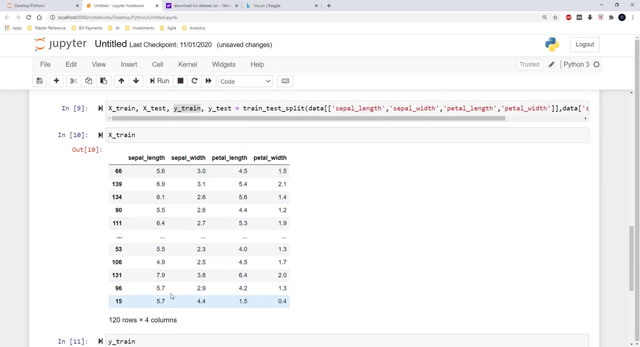 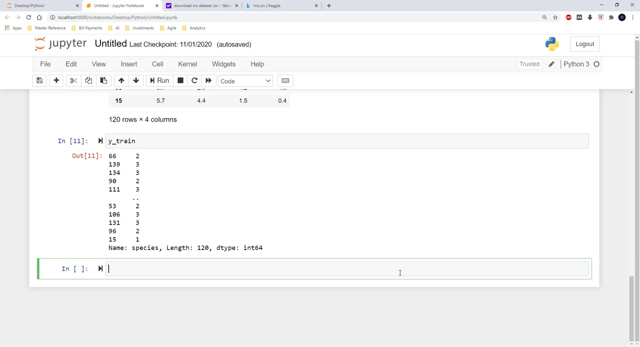 the x train. so this will be used for training and the x test and the y test will be used for testing and these two data sets will be having 30 rows. next, we are going to build the logistic regression model and we are going to use the x train and y train. 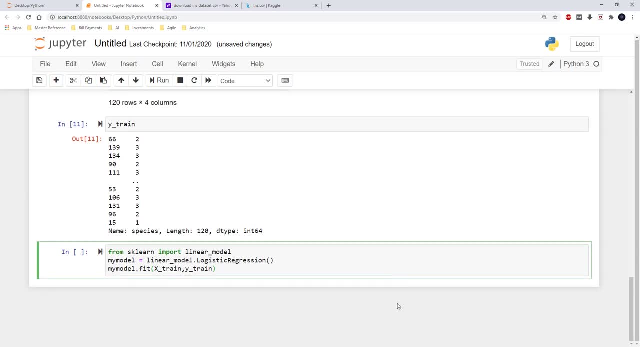 to train the model. so I am using this block of code here. I am importing linear model from sklearn and then I am creating an instant of logistic regression class and I am naming that instance as my model and then I am referring the method fit of logistic regression class. 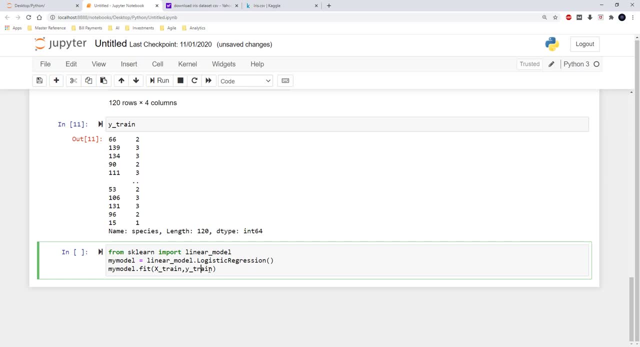 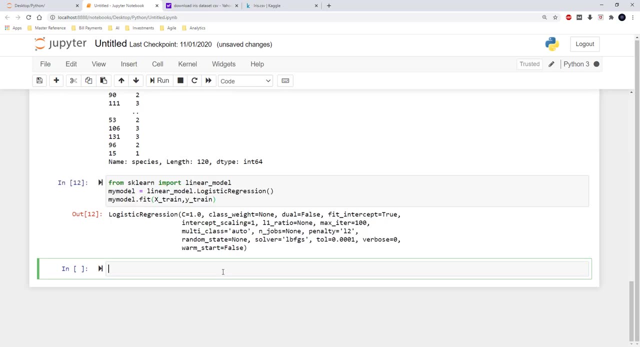 and I am giving the x train and y train as inputs to train the model and I am creating or running this block of code. you can see that the model has completed and sometimes you may get a error saying that the model has not converged and it will. the error message will ask: 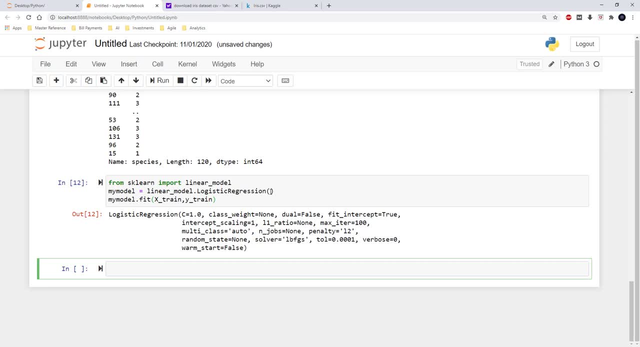 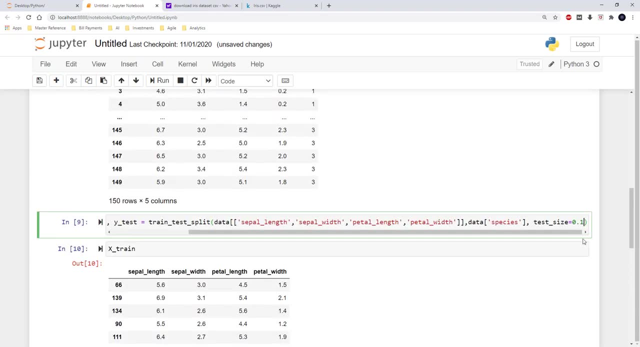 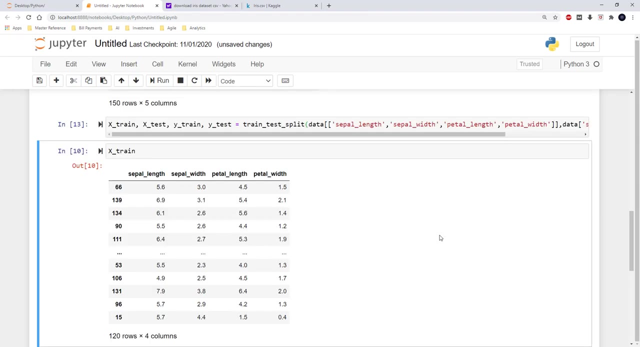 you to increase the maximum number of iterations. so here, in order to just demonstrate that error, I am going to have only 10 percent to test my data and the remaining 90 percent I am going to use as my training data. so I will run this block of code again and then x train is going to have 135 rows instead of 120. 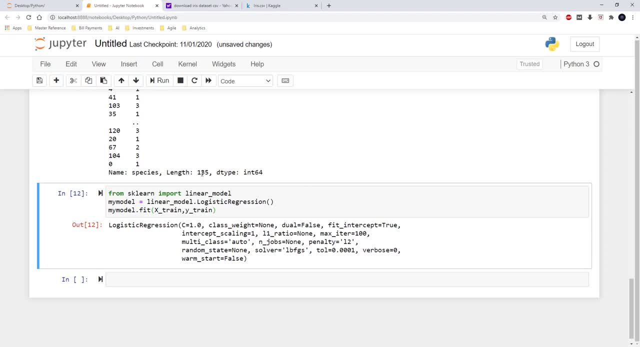 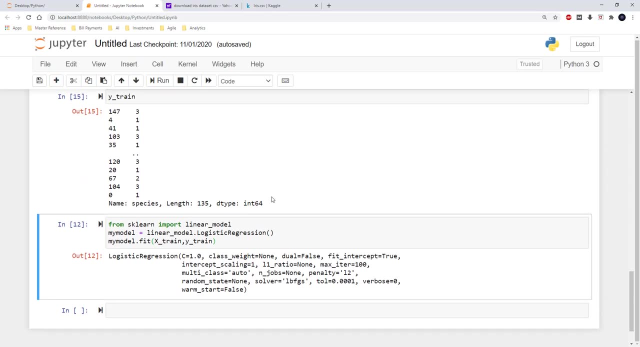 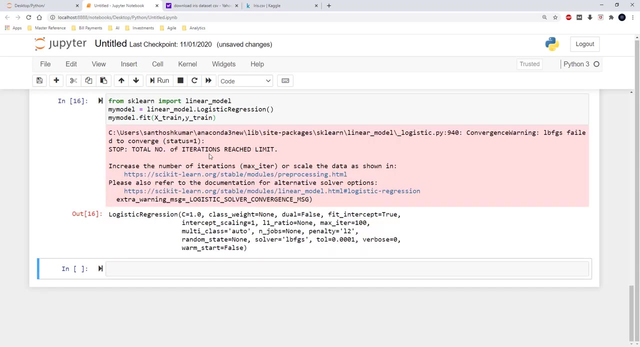 rows and y train is going to have the same 135 corresponding attributes for the dependent attributes. and now, when I run this model again, you can see that there is a error throwing up. so the error says that the convergence warning and the model has failed to converge. the total number of iterations has. 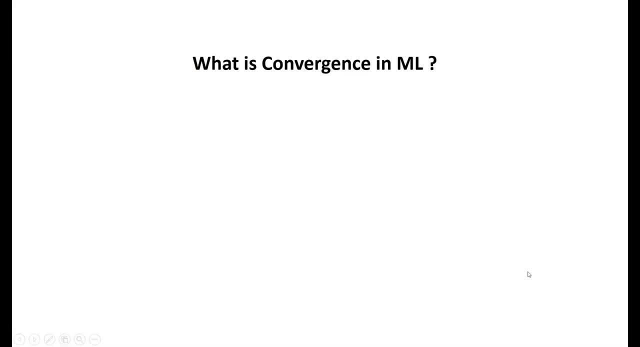 reached the limit. in order to understand the convergence convergence error, we need to understand what is convergence in machine learning. so what happens in machine learning is the model makes the predictions based on the input data that we are giving. in our case, we have given 135 rows. 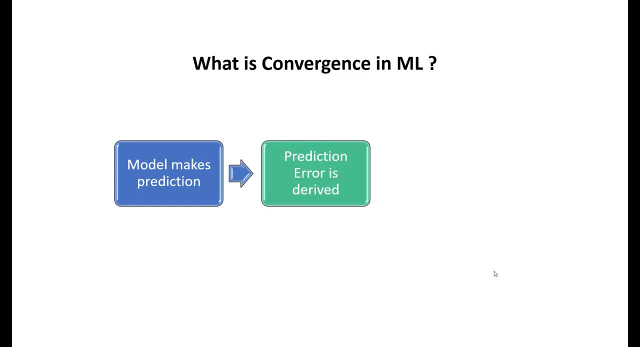 of test data and once the predictions is done, the model will check the predicted outcome with the actual outcome and then calculate the error. after the error is calculated, the model will try to minimize the error after each predictions and and this iteration is repeated until the error keeps minimizing once. 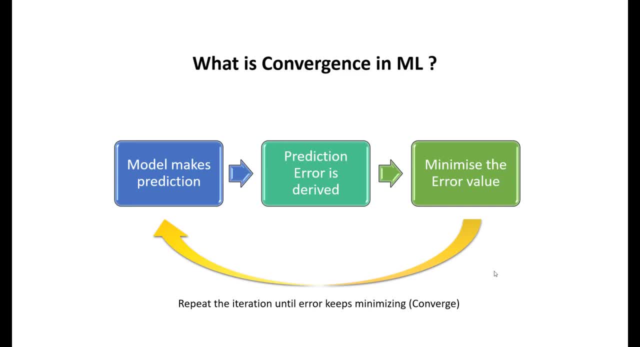 the error has reached its minimum value, then it means that the model has converged. after the model has converged, there will not be any possibilities of the model to further reduce its error. in our case, the model was trying to converge after each iterations, but it was not able to converge because 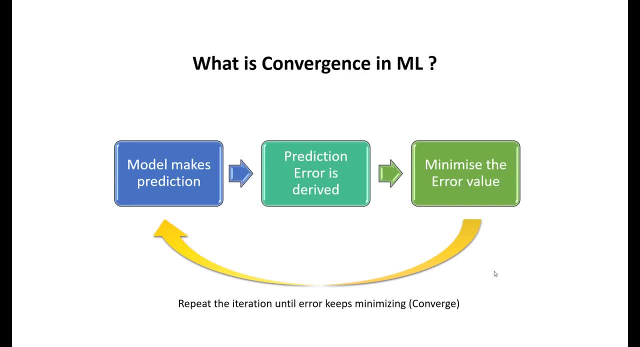 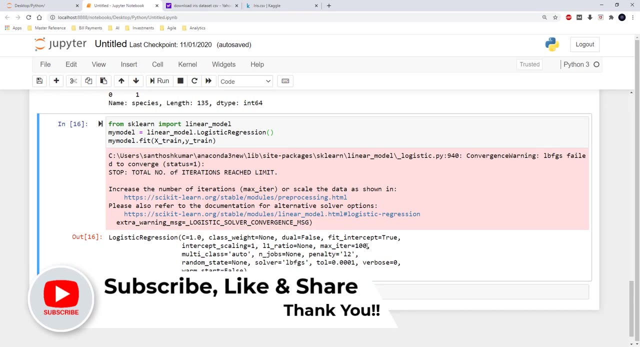 the preset value on the number of iterations has reached this limit. in order to resolve this error, we need to increase the maximum number of iterations. coming back to the code, the maximum number of by default is 100, and the 100 iteration was not enough for our model to converge. 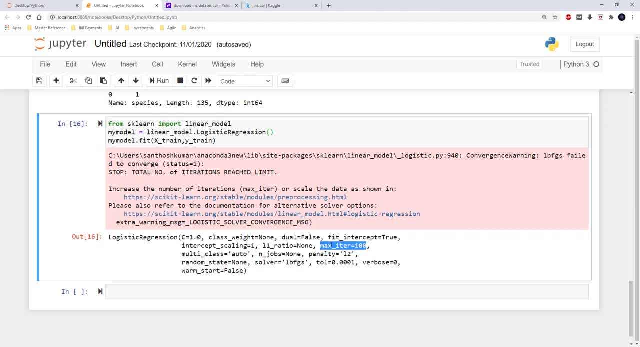 to a minimum error. so I am going to increase the maximum number of iterations. in order to do that, in the logistic regression class I am going to give this max underscore iter value to 120 and I am going to run this block of code again. when I run this again, you can see that the machine learning model has. 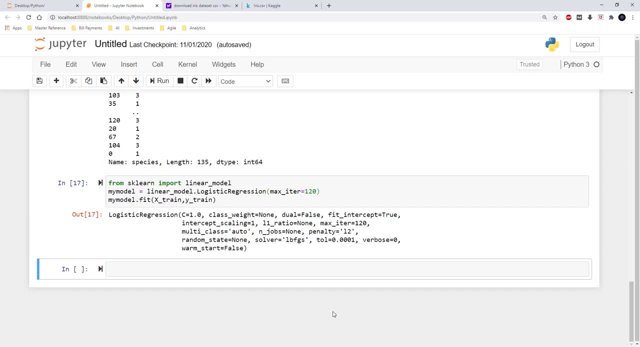 run without any errors. now I can use this model to make predictions. in order to do that, I am going to use my model dot predict, and here I am going to give the X test as input. when I run this block of code, you can see that the 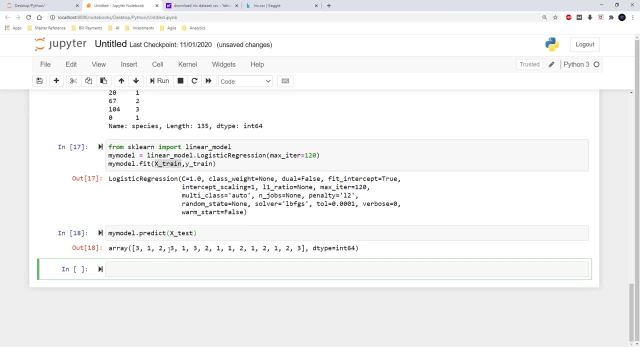 predictions has been done and there are around like 15 values or 15 outputs, and these outputs are the output values of the model and the output values are the predictions made by the model for the test data set. so just to have a feel of how the test data set looks like, I am going to print the test data set and you 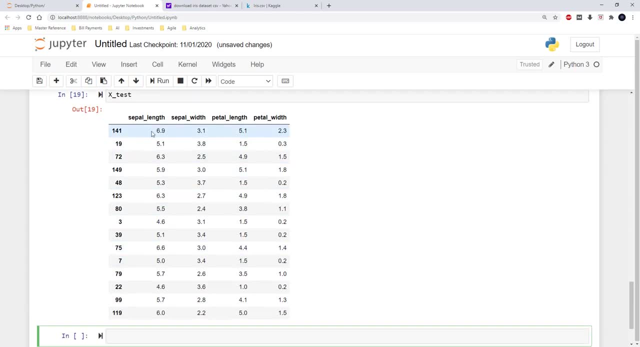 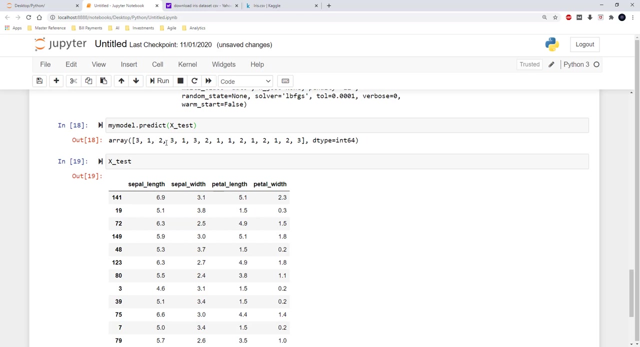 can see that these- and this is the test data set and it has totally 15 rows and each of this rows will be having independent attributes and for these independent attributes, or for the set of independent attributes, the model has predicted the outcome. so, for example, for this first set, the model has predicted. 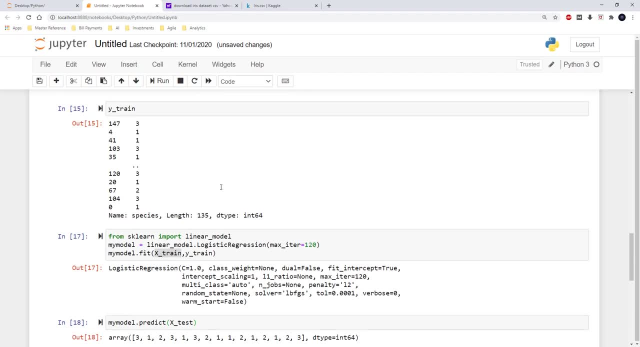 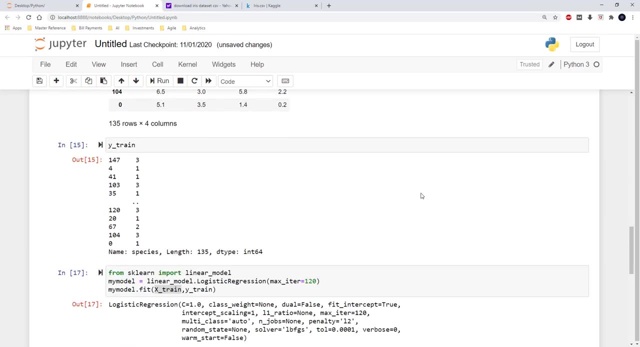 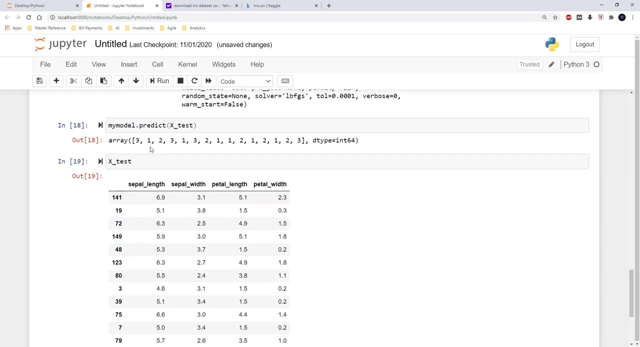 the outcome of three, which means that the species is actually Iris virginica, and for the second set of attributes, even independent attributes, the model has predicted the outcome of one, which means that the species is, or the collection plus h argument of one, which means that the species is affected more than one for each number. but you can see that one was predicted more than one. 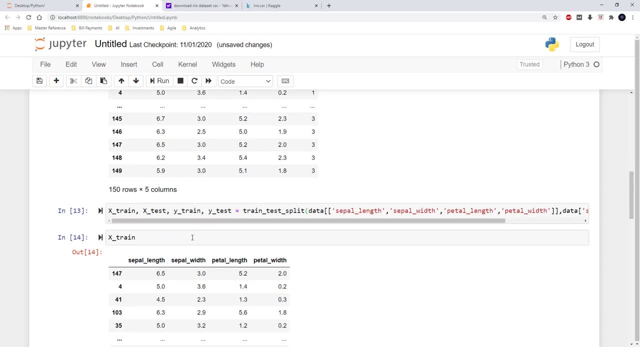 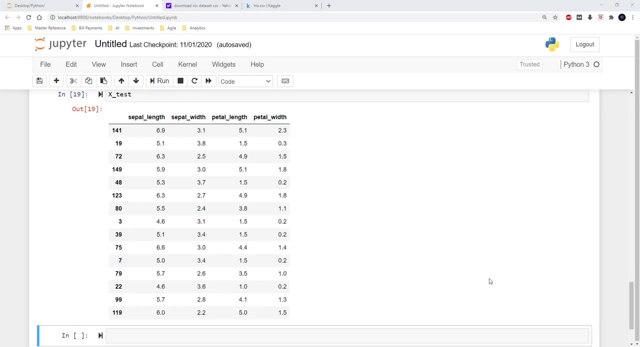 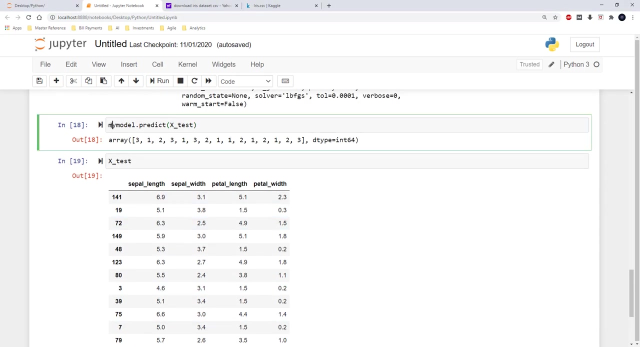 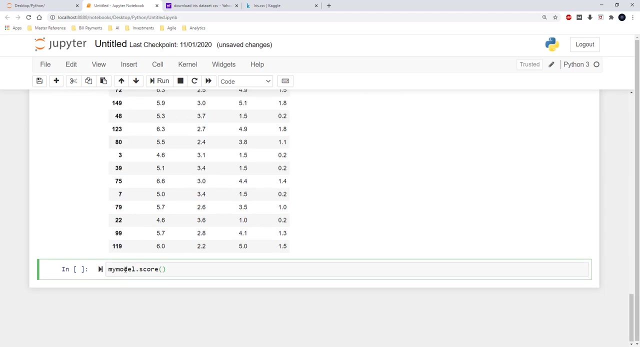 pred hoffe is iris setosa. likewise, the model has predicted the outcome for all the independent attributes. the model has made predictions, but we don't know how accurate it is. in order to know the accuracy of the model, I can use my model dot score and then I can give the test data set X, underscore test and Y. 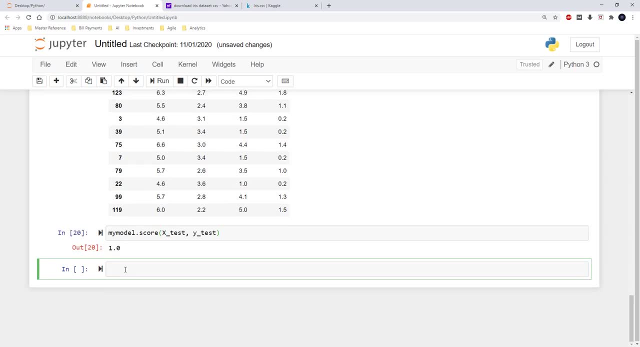 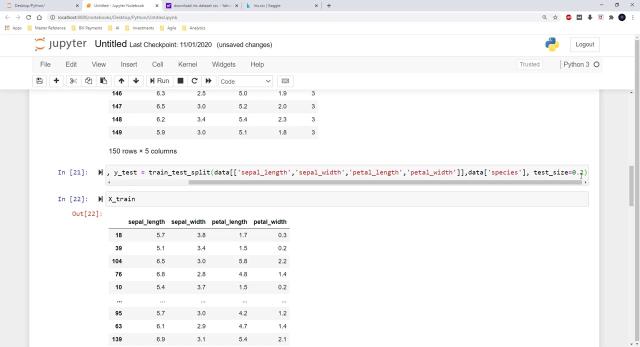 underscore test and get the score. and the score of my model is 1.0, which means my model is 100% accurate. I am just going to decrease my training data set and increase the testing data set, so I am going to give 30% of my data for. 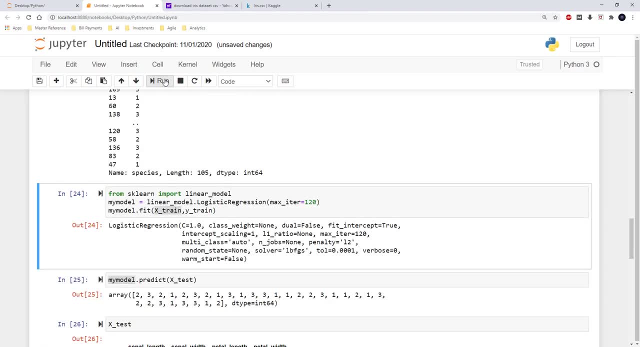 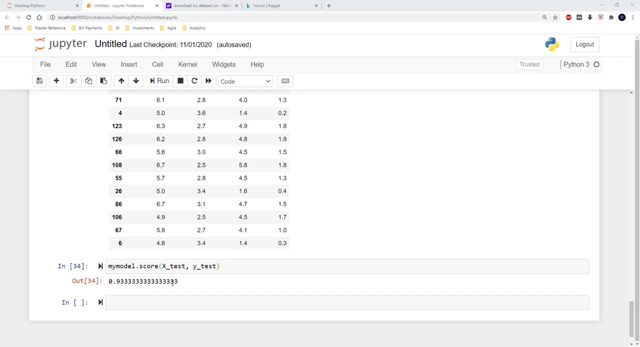 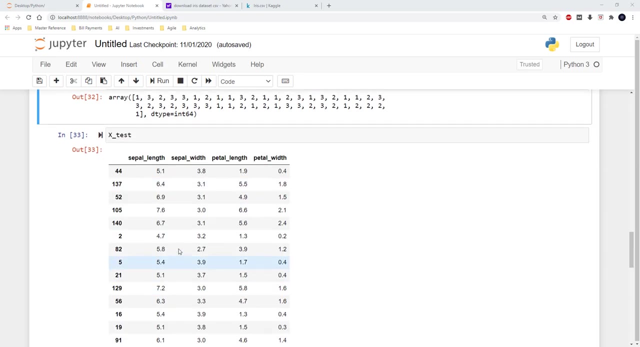 testing and the remaining for training, and I am going to rerun this block of code so that accuracy of our model now is 93.33%, and this is the outcome that is predicted by our model for the input, which is displayed over here. so we wanted to know. 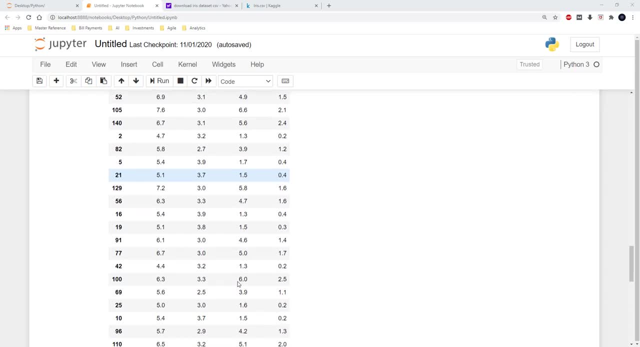 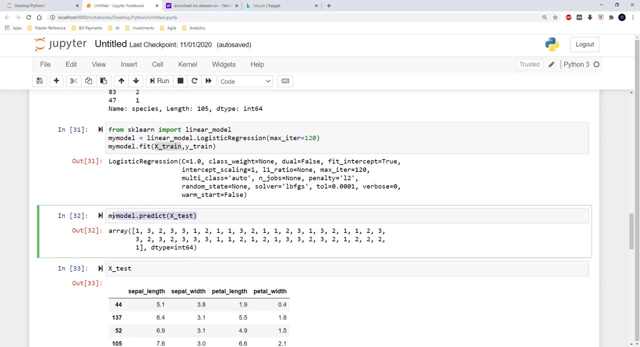 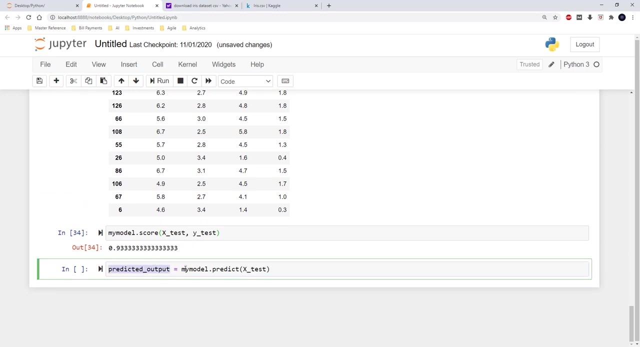 more about where this model has went wrong and in order to know that there is something called confusion matrix. so what I am going to do is I am going to just store the predicted output into a variable called predicted output, and when I display the predicted output, you. 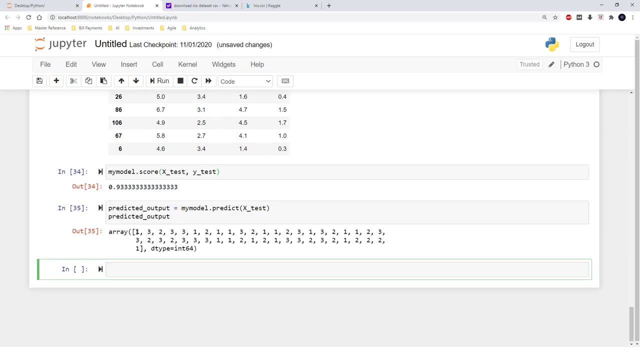 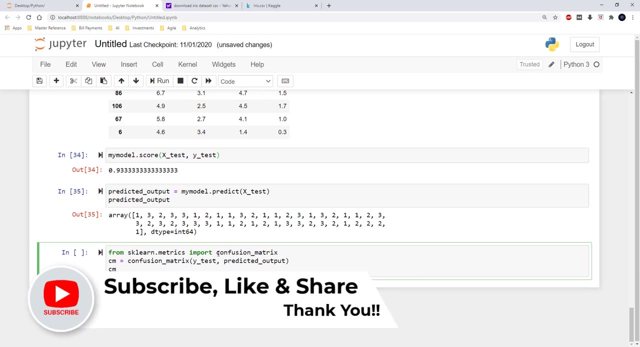 can see that it is a array and it is having all the outputs. that has been predicted by the model. next, I am going to use this block of code where I have imported confusion matrix from sklearnmatrix and then I am just creating CM, which is the instant of confusion matrix class, and I am going to 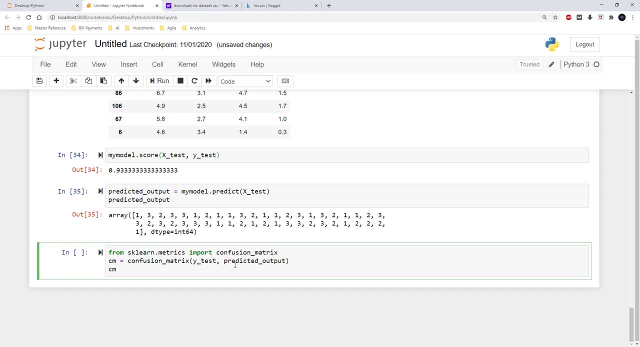 just serious t nothing. and for now we have passed y underscore test and predicted output. y underscore test is the actual output and here we have the predicted output and for both the actual output versus the predicted output. I am all theaa self a. I mean creating the confusion matrix and I am displaying the matrix. so 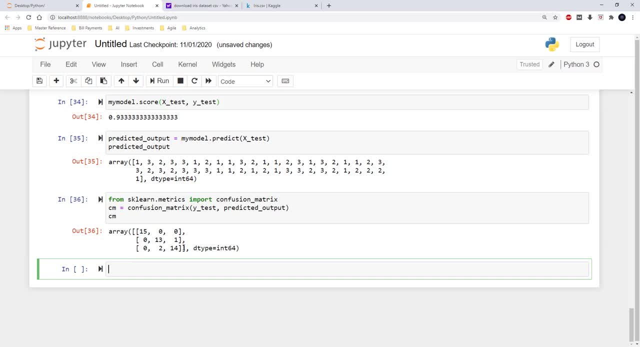 when it displayed the value of CM. you can see that a 3 by 3 either is created, and know at this point of time is that there are three possible outcomes that our model can predict, and hence we have got a 3x3 array. 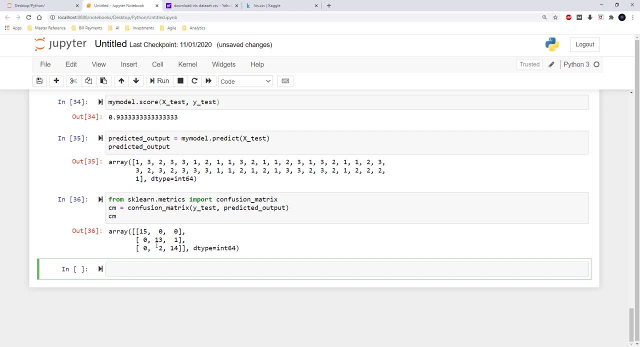 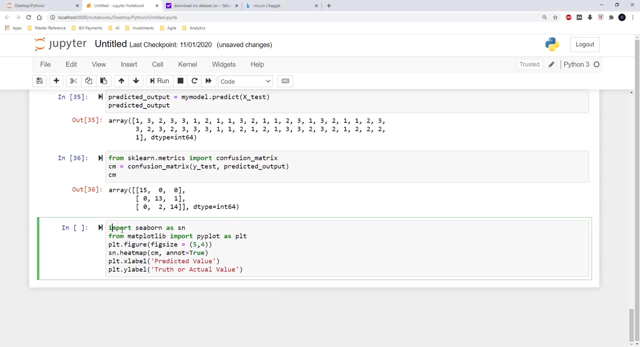 But you may just be thinking: what does this actually signifies? In order to explain that better, I am going to use a seaborn plot. In order to explain this confusion, matrix array better, I am going to use this block of code where I am importing seaborn as sn and I am importing pyplot from matplotlib. 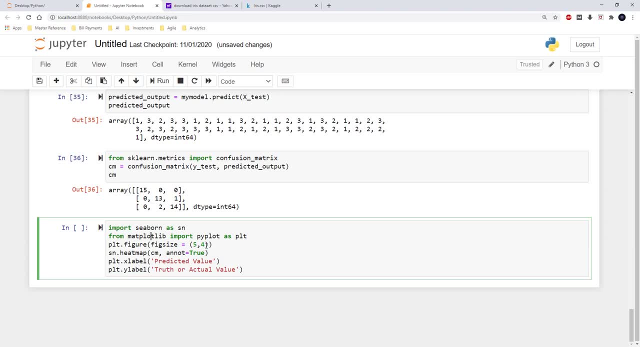 and I am using the plot size or figure size as 5x4, which means x axis the size is 5 and y axis the length is 4.. And then I am using seabornheatmap and I am giving the confusion matrix as input. 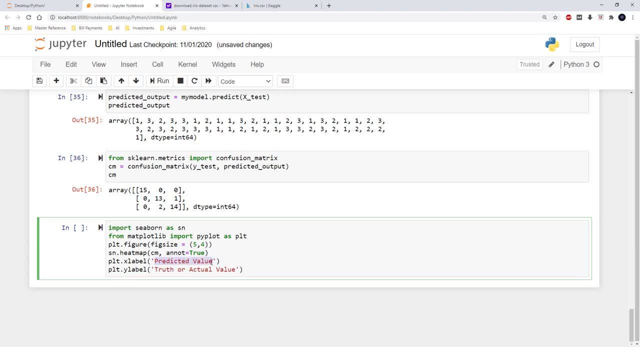 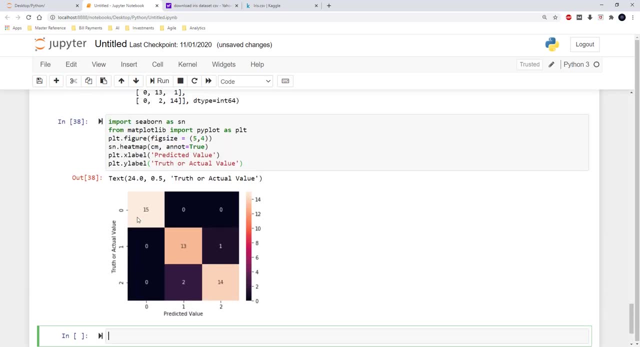 And I am labeling this, Using the x axis as predicted value and y axis as truth or actual value. And when I run this block of code, you can see that this plot is generated and here, in the x axis, we have the predicted value by the model and in the y axis, we have the actual. 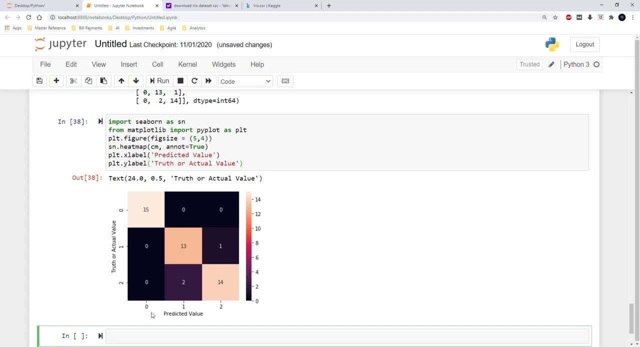 value or the truth. So what this plot means is: the model has predicted 0, where the actual value as well was 0 and the actual value as well was 0, and this has happened 15 times, and this credit correct prediction has happened 14 times, but one time the model 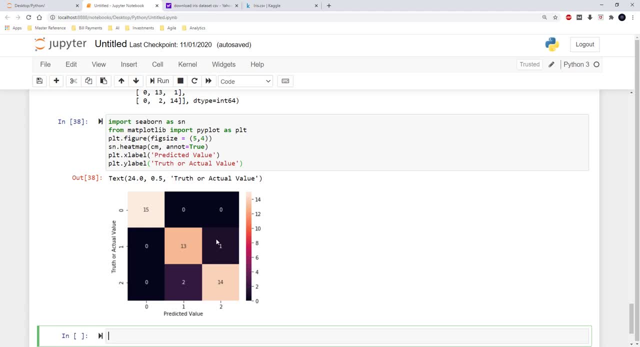 has predicted the value of 2 where the actual value was 1, and this is wrong. so you can see that out of the total 45 predictions, 3 has went wrong and this is how the wrong predictions was made, and this is the use of confusion matrix. so 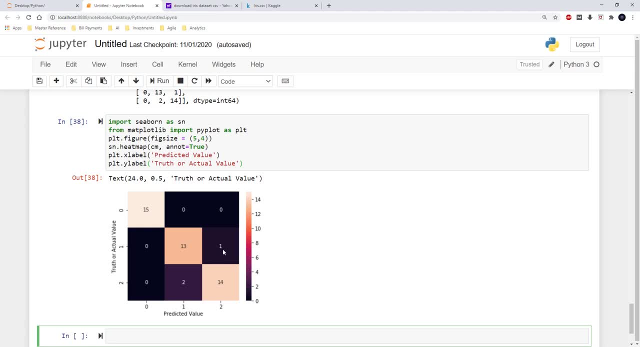 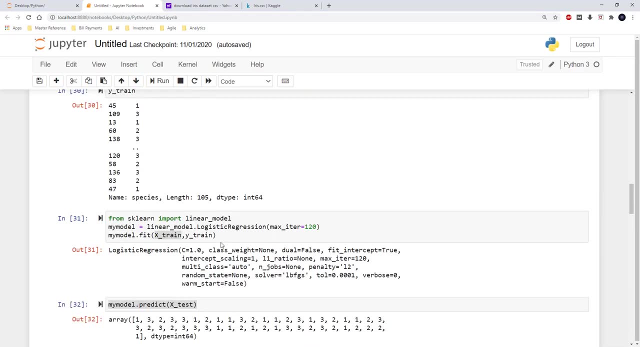 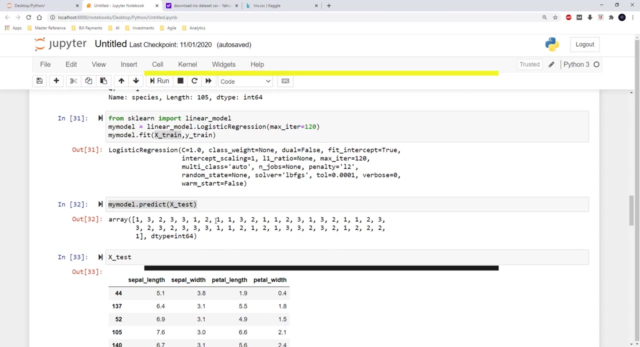 this is all I have for this video. you can refer the description of this video and I have included the link for this code and, and in the description of the video I have included the links of my all the other videos. please have a look and I hope you like this video, if you have not already subscribed to my 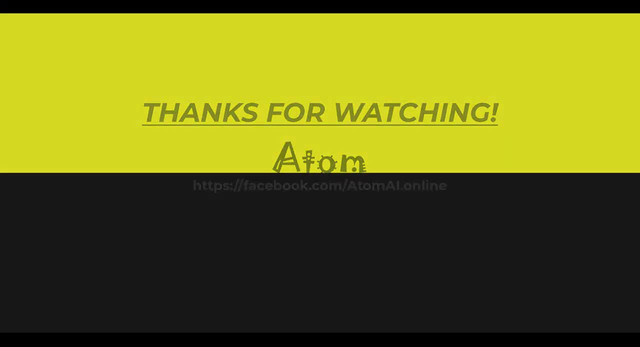 channel. please subscribe it. thank you very much.